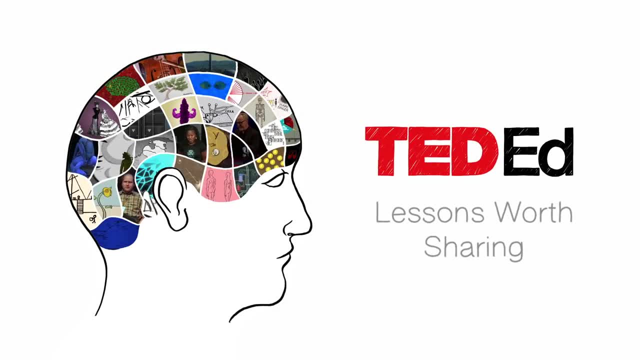 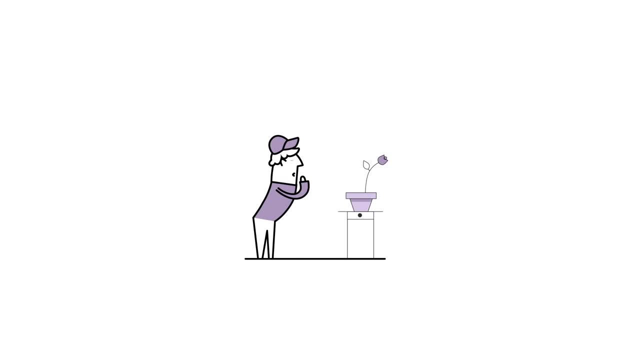 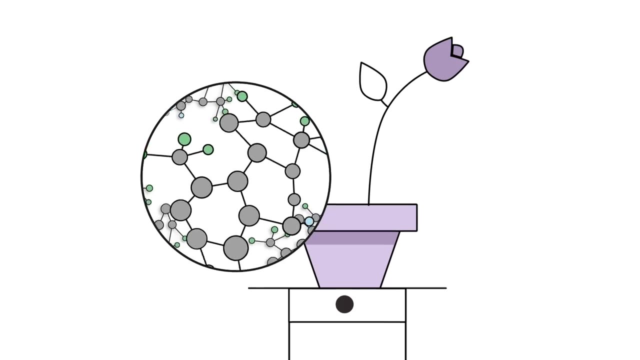 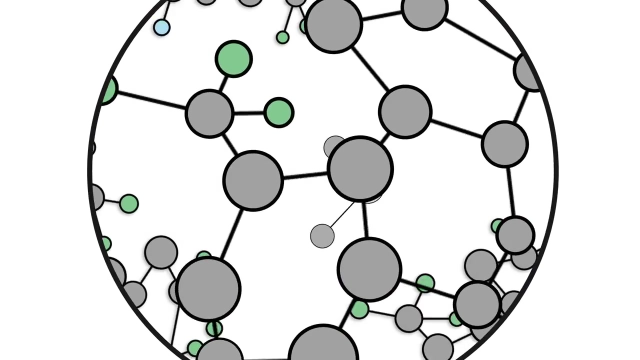 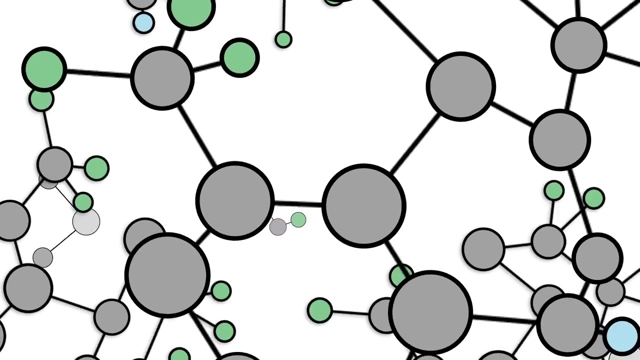 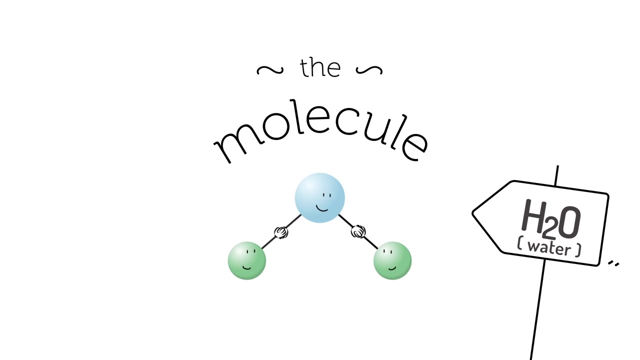 We'll see you next time on Inanimate Objects- And that describes almost all substances- Move according to a set of principles. For example, take molecules, atoms held together by covalent bonds. There are three basic ways molecules can move: Rotation, translation and vibration. 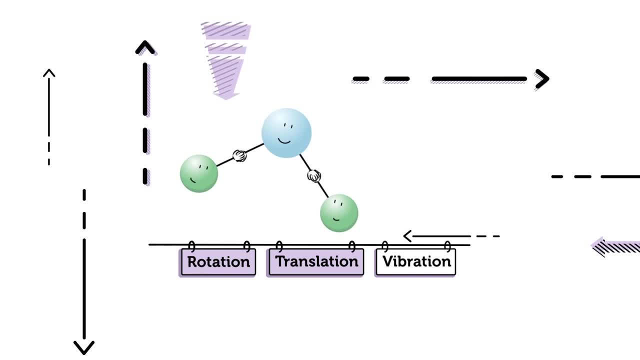 Rotation and translation move a molecule in space while its atoms stay the same distance apart. Vibration, on the other hand, changes those distances, actually altering the molecule's shape. For any molecule, you can count up the number of different ways it can move. 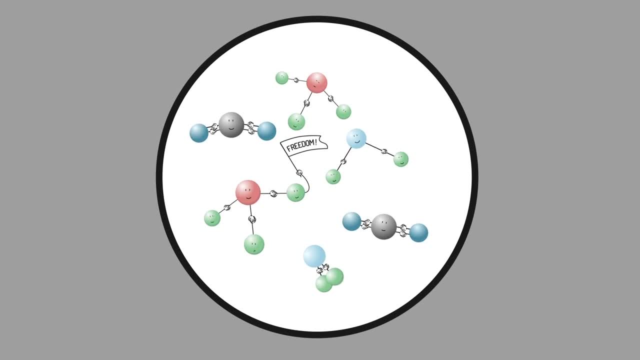 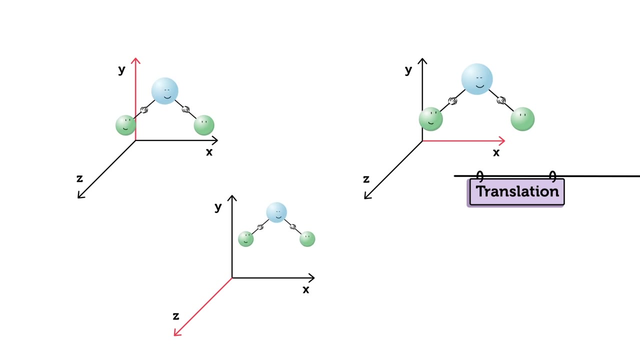 That corresponds to its degrees of freedom, which, in the context of mechanics, basically means the number of variables we need to take into account to understand the full system. Three-dimensional space is defined by x, y and z axes. Translation allows the molecule to move in the direction of any of them. 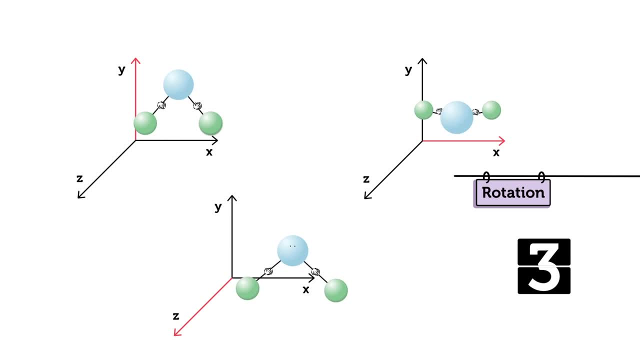 That's three degrees of freedom. It can also rotate around any of these three axes- That's three more- Unless it's a linear molecule like carbon dioxide. There, one of the rotations just spins the molecule around its own axis, which doesn't count because it doesn't change the position of the atoms. 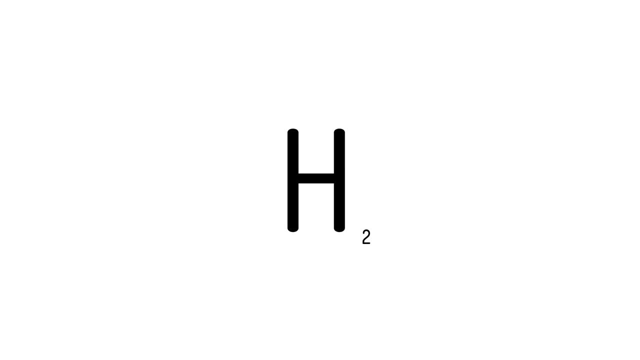 Vibration is where it gets a bit tricky. Let's take a simple molecule like hydrogen. The length of the bond that holds the two atoms together is constantly changing, as if the atoms were connected by a spring. That change in distance is tiny, less than a billionth of a meter. 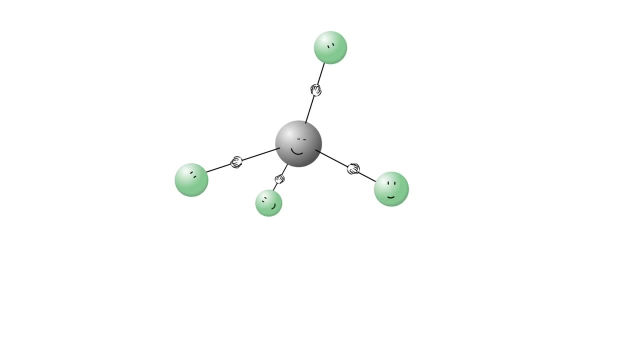 The more atoms and molecules are connected, the smaller the distance. The more atoms and bonds a molecule has, the more vibrational modes. For example, a water molecule has three atoms, one oxygen and two hydrogens, and two bonds. That gives it three modes of vibration. 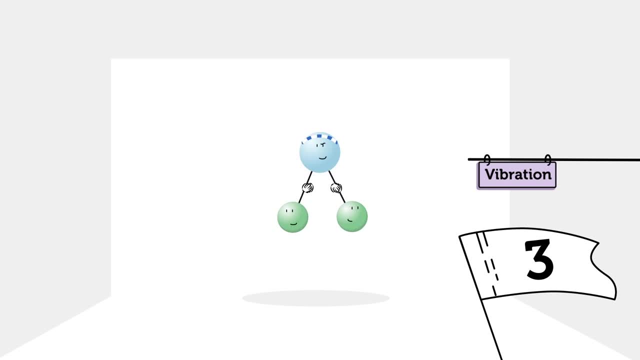 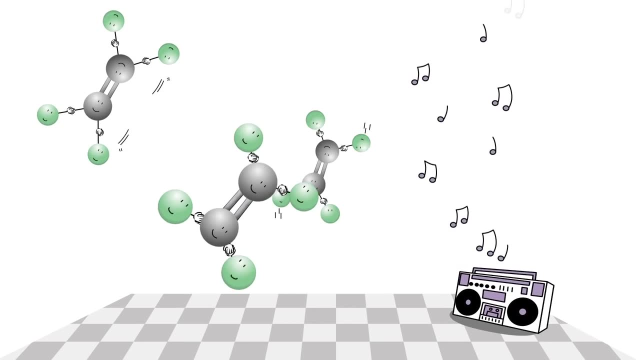 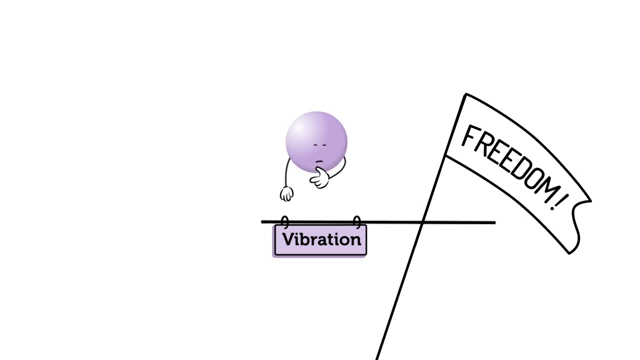 symmetric stretching, asymmetric stretching and bending. More complicated molecules have even fancier vibrational modes like rocking, wagging and twisting. If you know how many atoms a molecule has, you can count its vibrational modes. Start with the total degrees of freedom.